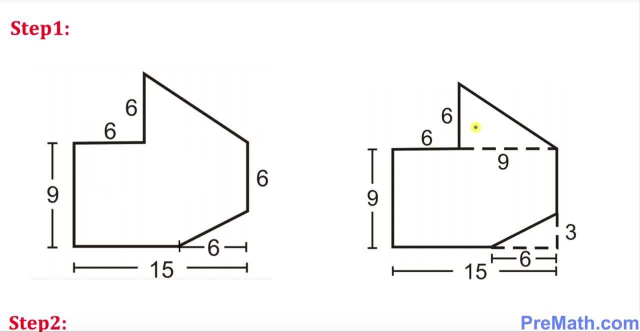 this given shape into three simpler regions. So you can see right now as I, because you can see that I have divided up into this one. this is over here. if you look at this one, this is a top triangle, and then we have this one is a rectangle, and then we have another right triangle. 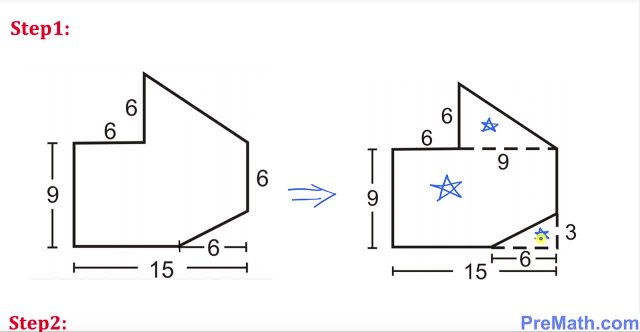 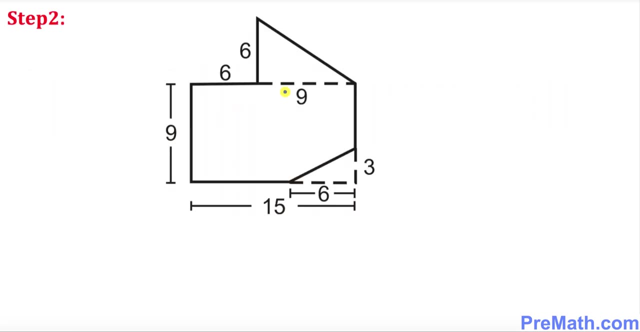 so we have a bigger triangle on the top and then smaller at the bottom, and then we have a rectangle. so we're gonna now find the area of these three individual shapes. and in this next step, before we find the area of these individual shapes, we want to find the formula to figure out the total area. 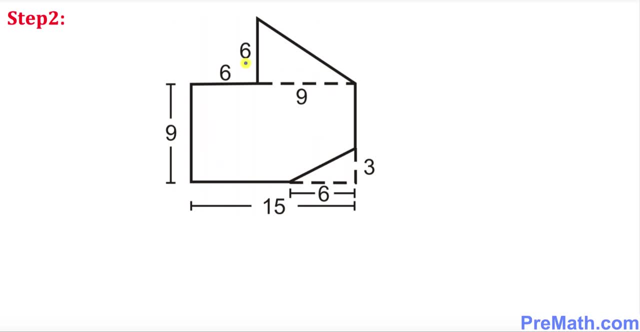 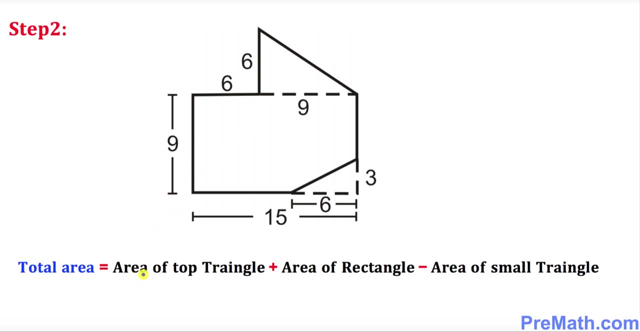 of this shape and this is the formula we will be using, and the total area of this given shape is gonna be equal to area of this top triangle. okay, this is the one area of the top triangle plus the area of this rectangle, and now this part is excluded, so no wonder I put down minus the 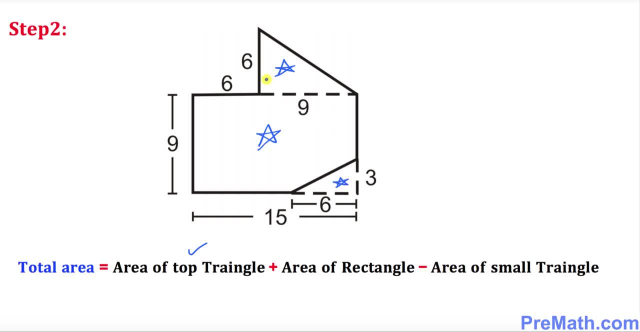 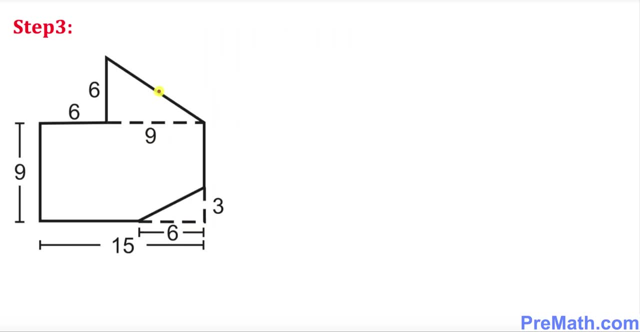 area of this rectangle, and now this part is excluded. so no wonder I put down minus the area of this rectangle, and now this part is excluded. so no wonder I put down minus the area of this rectangle, of this small triangle. these are, by the way, these two triangles are right triangles. and in this next, 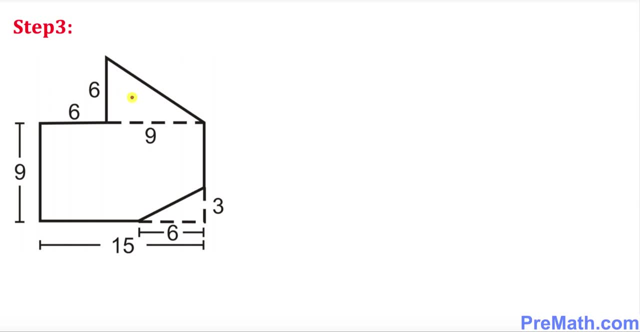 step. let's go ahead and find the area of these two right triangles. we're going to be finding the area of these two right triangles and the formula to find the area of these triangle is is right up here. the area equals to a half time base time height in this triangle. this side is our base. 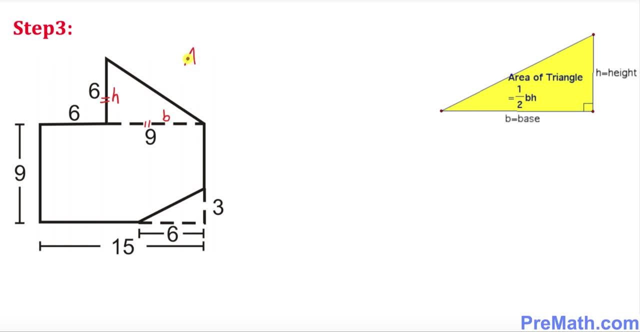 this side is our height, so area equals to a half time. base is nine times height is six. let's go ahead and multiply it out, so that's gonna be simply seven. so the area of this turns out to be 27 square units. so, similarly, we're going to be: 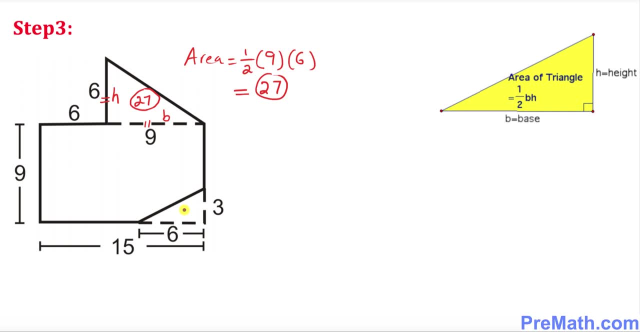 finding the area of this right triangle as well over here. this is our base. this is our height we will be using once again. so the area equals to a half times base is six and the height is three. when you multiply it out and divide by two, that's gonna be nine. so the area of this triangle turns out to be: 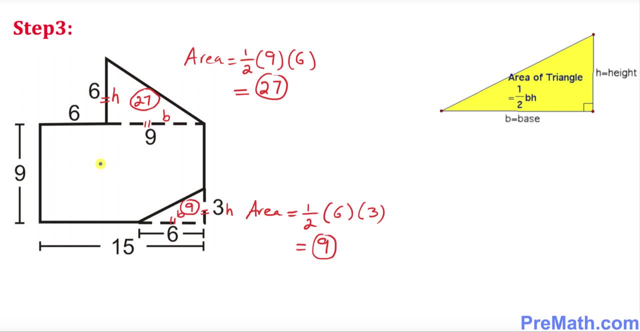 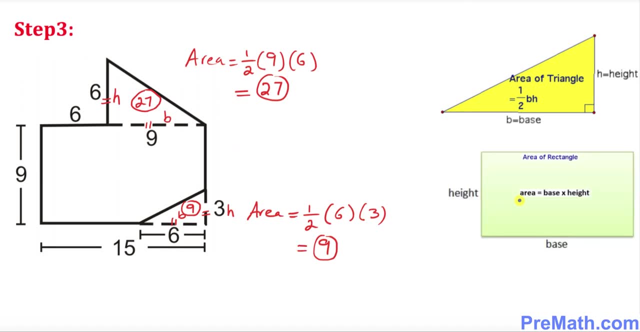 nine. and finally we now argue: are we going to find the area of this rectangle? and the formula is: as you can see, the area of a rectangle is always equal to base time height. as you can see, the base is 15 and the height is 9 of this rectangle, so that means the 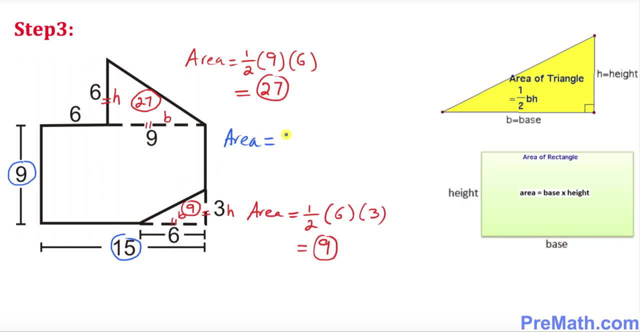 area is going to be a: simply base is 15 times height is 9 means we got 135.. so that means the base is 15 and the height is 100, so this is gonna be base area. y is gonna be a: simply base is 15 times height is nine means we got. 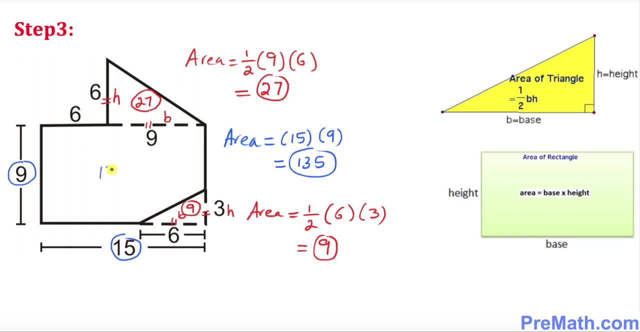 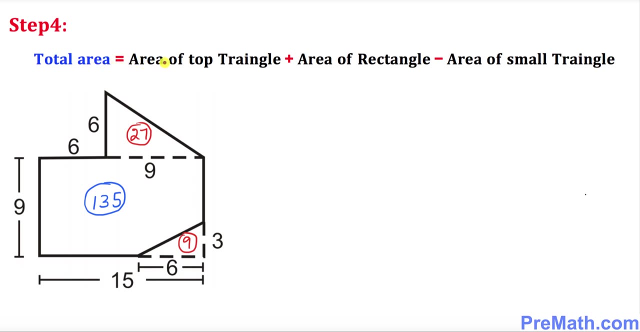 135. so that means the area is gonna be a. simply, base is 15 times height is 9. that means we got 135.. 135 so that means 135 is the area of this rectangle and in our final step we are going to plug it in everything in our formula. okay, the area of the top triangle we figured out was 27.